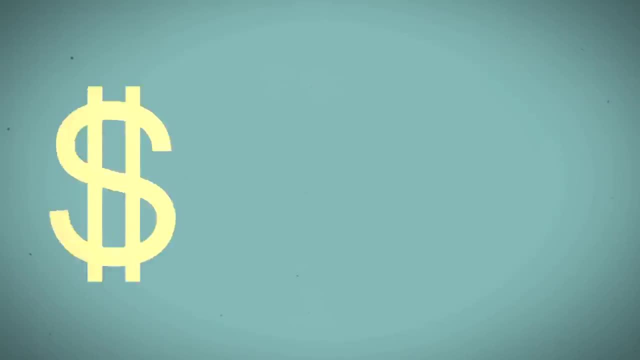 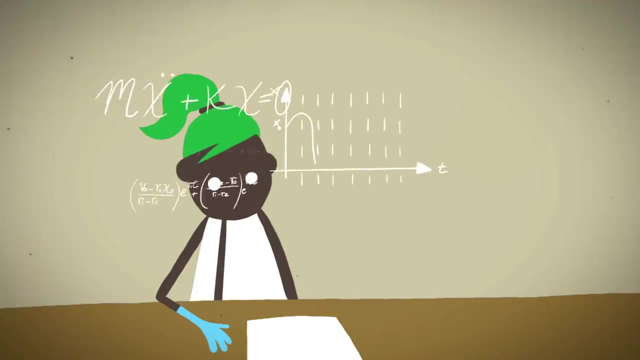 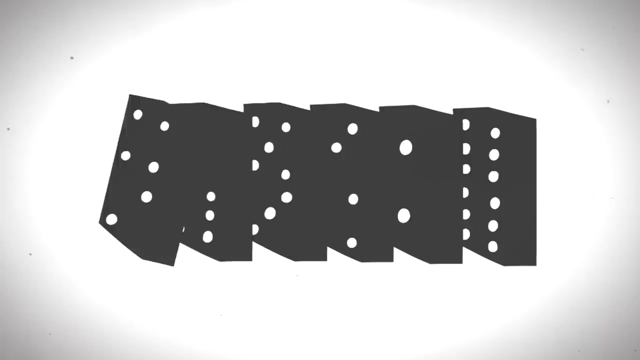 It turns out, nuclear power faces many hurdles, including high construction costs and public opposition, And behind these problems lie a series of unique engineering challenges. Nuclear power relies on the fission of new nuclear solutions, which make it difficult to build systems that will sustainability. 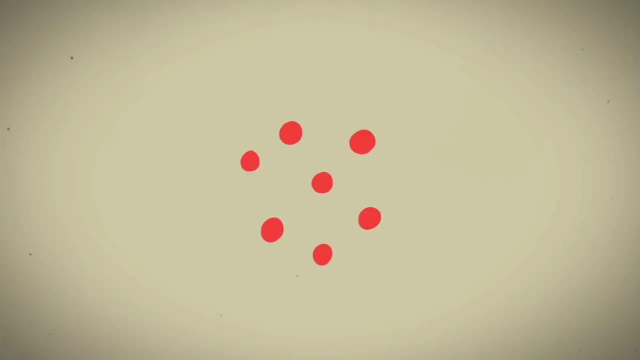 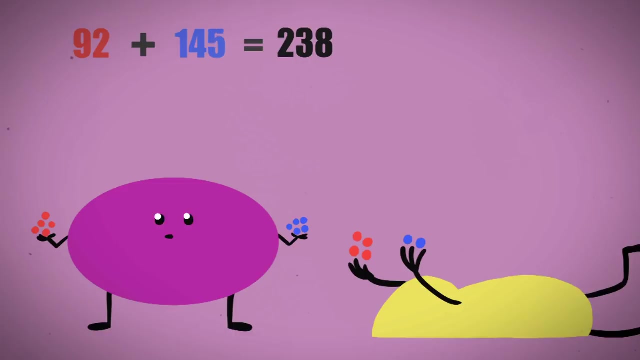 Clothing for nuclear energy can be used by the industry to often go in the wrong direction. But thanks to nuclear power we can become a more efficient world And that's why the nuclear nuclear power plant is almost unique in 150 ways. The nuclear nuclear power plant. 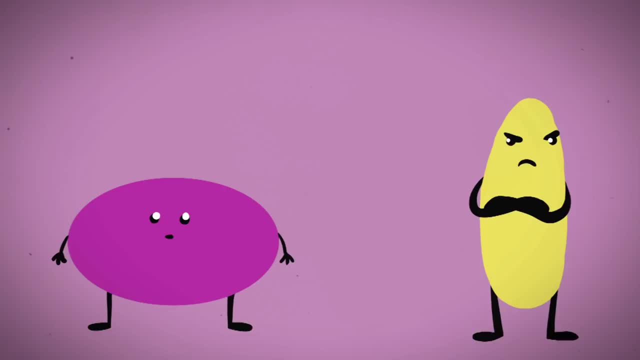 is the largest nuclear power plant in the world. with the largest nuclear power plant in the world and is the largest nuclear power plant in the world. a strike by a neutron easily splits the U-235 nuclei into lighter radioactive elements called fission products. 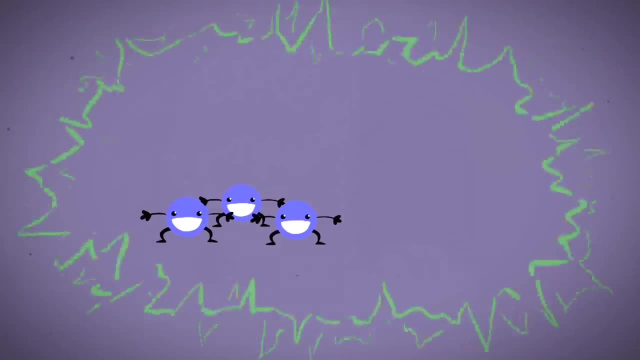 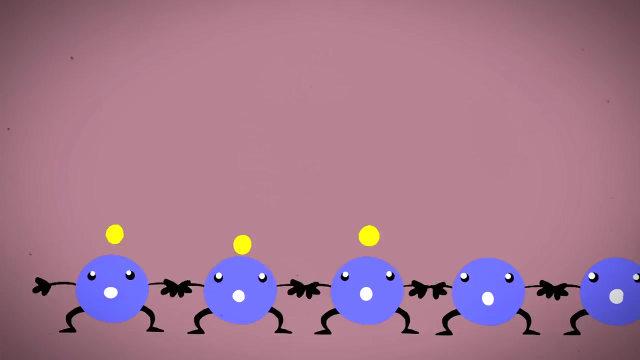 in addition to two to three neutrons, gamma rays and a few neutrinos. During fission, some nuclear mass transforms into energy, A fraction of the newfound energy powers, the fast-moving neutrons and, if some of them strike uranium nuclei. fission results in a second, larger generation of neutrons. If this second generation of neutrons strike more uranium nuclei, more fission results in an even larger third generation, and so on. But inside a nuclear reactor this spiraling chain reaction is tamed using control rods. 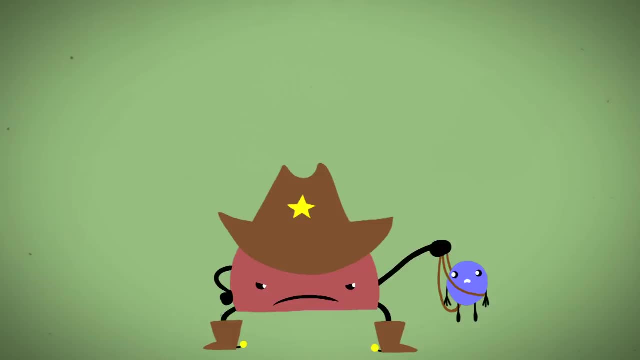 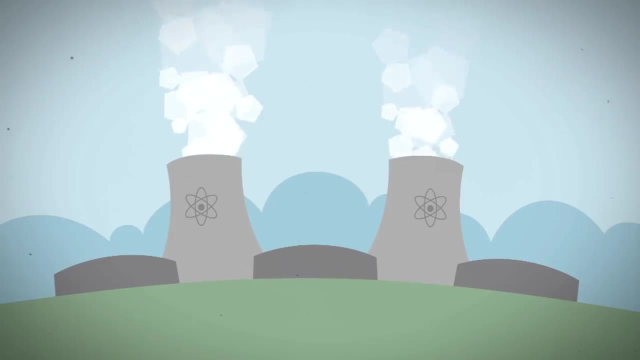 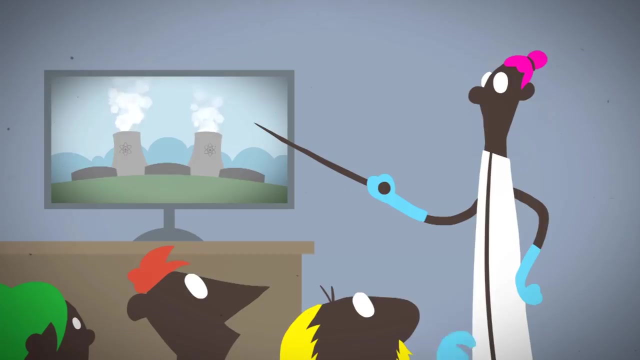 made of elements that capture excess neutrons and keep their number in check. With a controlled chain reaction, a reactor draws power steadily and stably for years. The neutron-led chain reaction is a potent process driving nuclear power, but there's a catch that can result in unique demands. 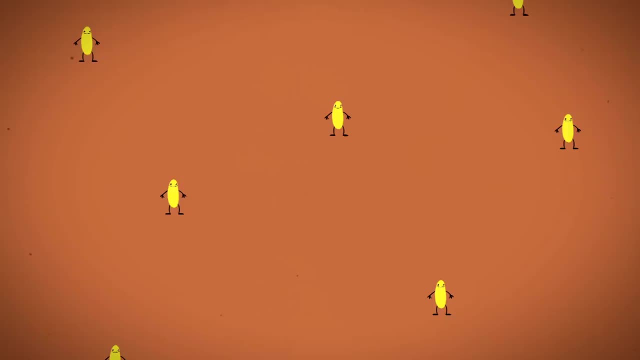 on the production of its fuel. It turns out most of the neutrons emitted from fission have too much kinetic energy to be captured by uranium nuclei. The fission rate is too low and the chain reaction fizzles out. The first nuclear reactor built in Chicago. 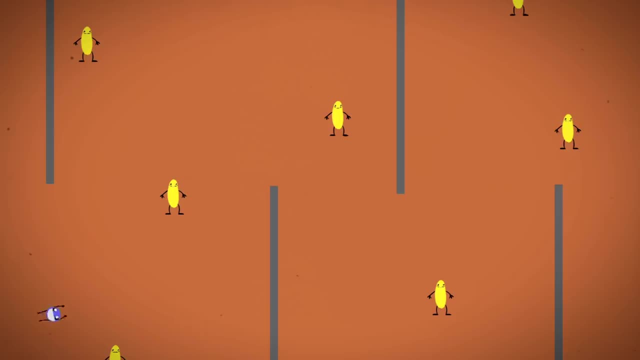 used graphite as a moderator to scatter and slow down neutrons just enough to increase their capture by uranium and raise the rate of fission. Modern reactors commonly use purified water as a moderator, but the scattered neutrons are still a little too fast. 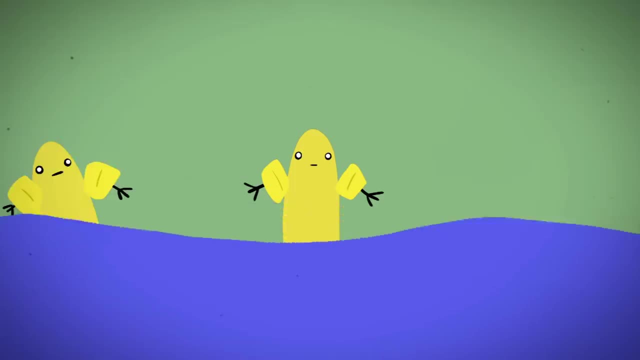 To compensate and keep up the chain reaction, the concentration of U-235 is enriched to four to seven times its natural abundance. Today, enrichment is often done by passing a gaseous uranium compound through centrifuges to separate lighter U-235 from heavier U-238. 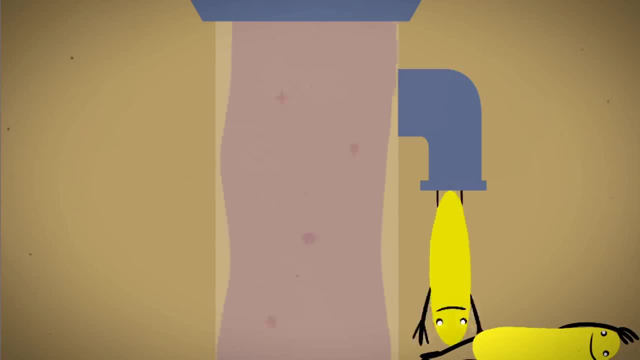 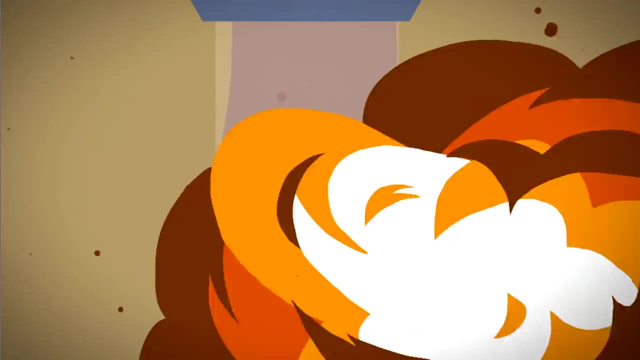 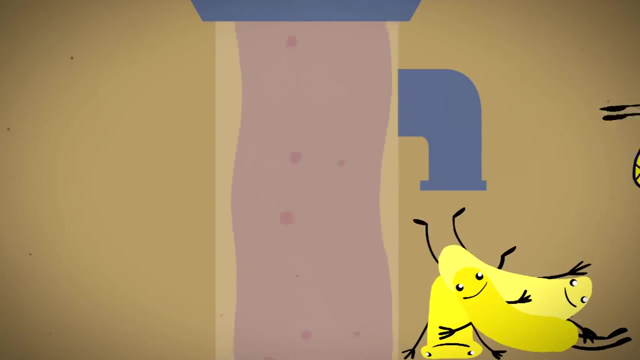 But the same process can be continued to highly enrich U-235 up to 130 times its natural abundance and create an explosive chain reaction in a bomb. Methods like centrifuge processing must be carefully regulated to limit the spread of bomb-grade fuel. Remember only a fraction of the released fission energy. 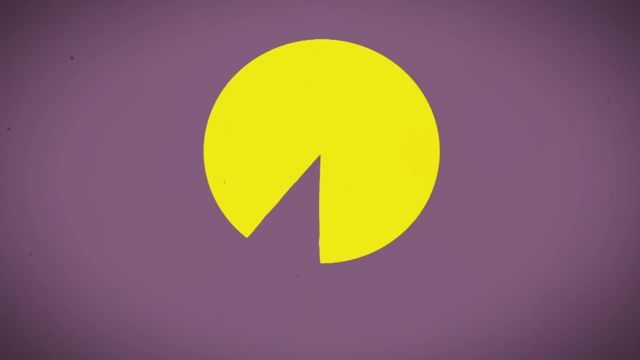 goes into speeding up neutrons. Most of the nuclear power flows into the kinetic energy of the fission products. Those are captured inside the reactor as heat by a coolant, usually purified water. This heat is eventually used to drive an electric turbine generator by steam. 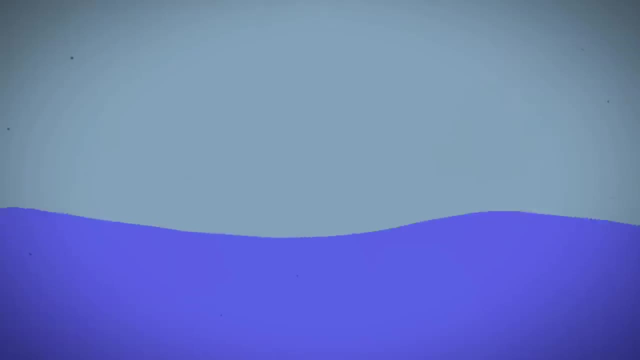 just outside the reactor. Water flow is critical not only to create electricity, but also to guard against the most dreaded type of reactor accident: the meltdown. If water flow stops because a pipe carrying it breaks or the pumps that push it fail, the uranium heats up very quickly and melts. 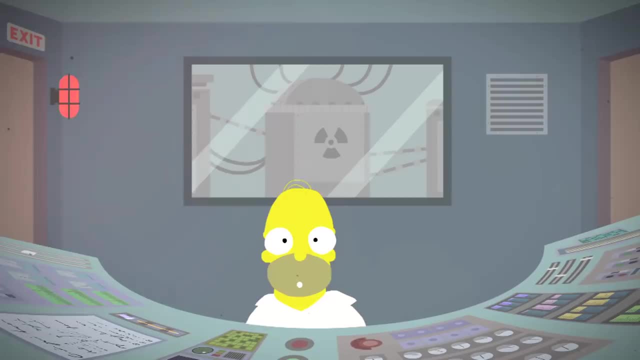 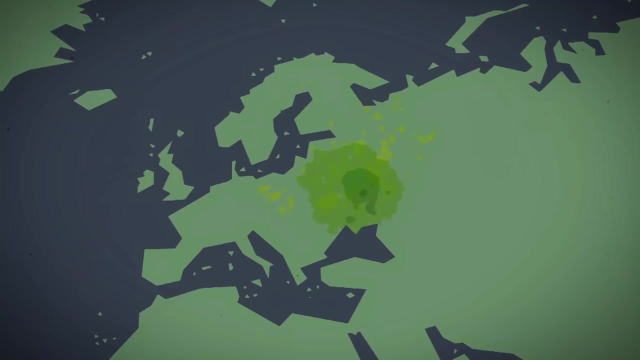 During a nuclear meltdown, radioactive vapors escape into the reactor, and if the reactor fails to hold them, a steel and concrete containment building is the last line of defense, But if the radioactive gas pressure is too high, containment fails and the gases escape into the air. 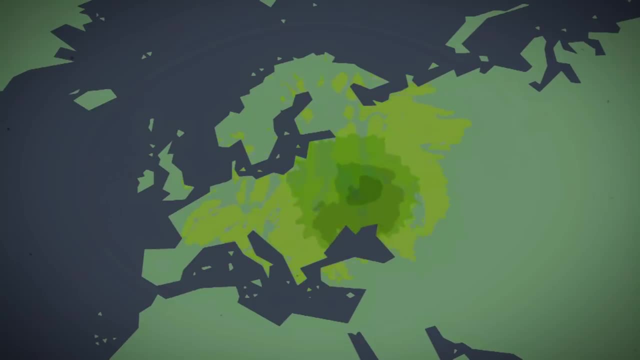 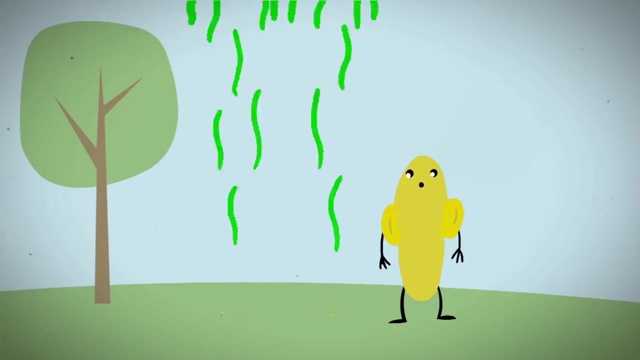 spreading as far and wide as the wind blows. The radioactive fission products in these vapors eventually decay into stable elements. While some decay in a few seconds, others take hundreds of thousands of years. The greatest challenge for a nuclear reactor is to safely contain these products. 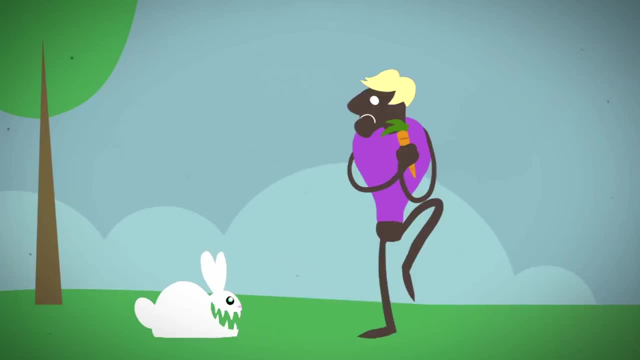 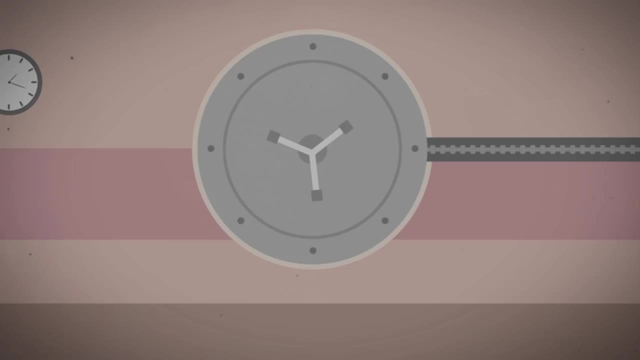 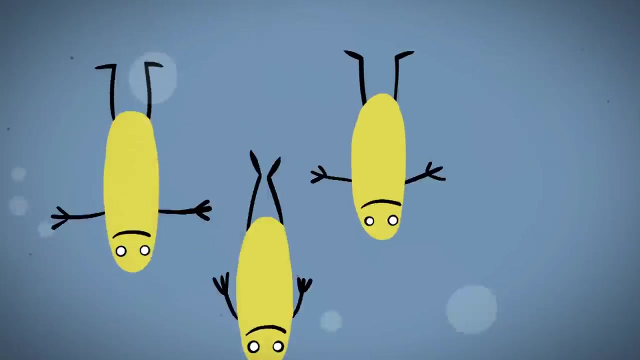 and keep them from harming humans or the environment. Containment doesn't stop mattering once the fuel is used up. In fact, it becomes an even greater storage problem. Every one to two years, some spent fuel is removed from reactors and stored in pools of water.